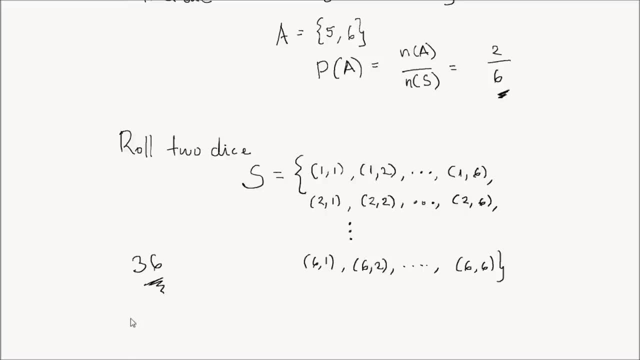 So you can imagine you could have experiments with thousands or maybe millions of elements in them. The goal of this lecture is to study methods of finding the number of elements in a sample space or in an event without the need to list all the elements. And the first method we 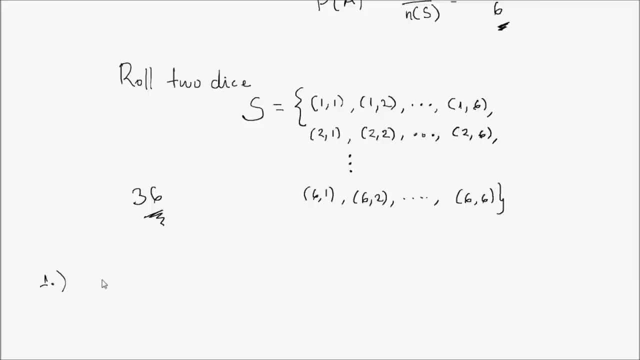 will look at is multiplication rule of counting. I will explain multiplication rule of counting with a very simple example. Consider yourself going to a very small restaurant, maybe in a very small town, which has only 3 appetizer choices and 2 main courses. So you could choose from 3 appetizers and 2 main courses. So you 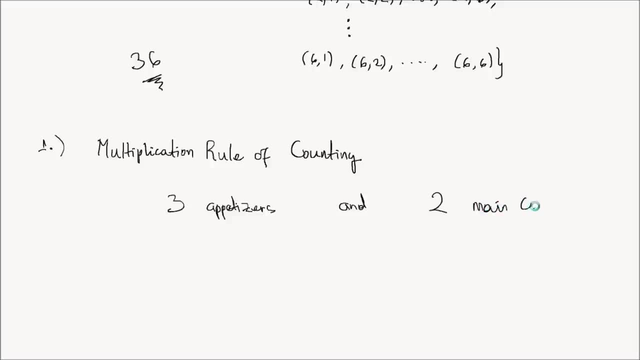 have 2 main dishes, main courses, And how many ways can you choose a meal? Of course you can choose appetizer 1, or maybe you want to choose appetizer 2, or maybe appetizer 3.. You have 3 choices Once you choose the 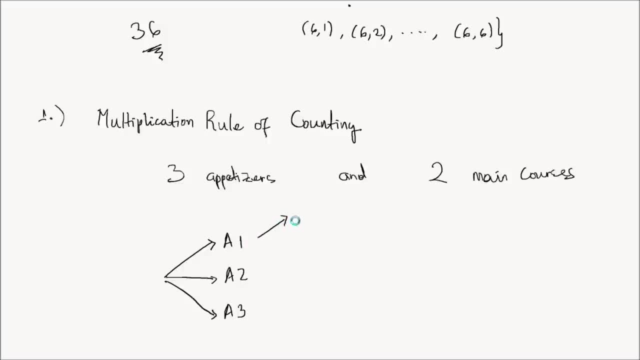 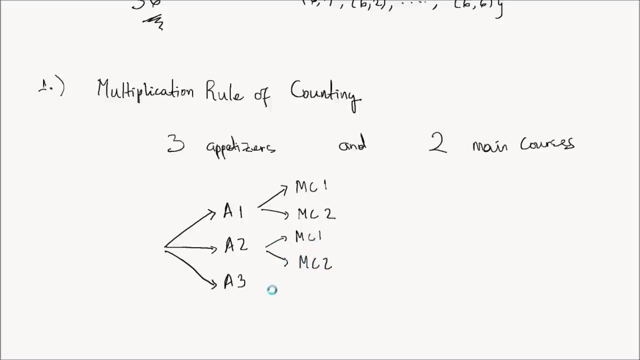 first appetizer. you can combine it with main course 1 or main course 2.. You can have it with the second main course. Likewise, you can have appetizer 2 with main course 1 or appetizer 2 with main course 2. 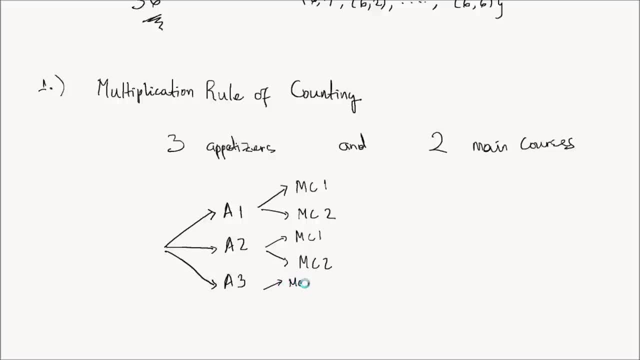 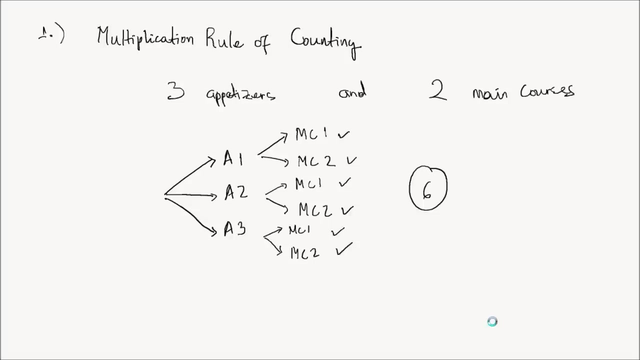 you can have appetizer 3 with main course 1 or appetizer 3 with main course 2.. Therefore, you get a total of 6 different possible ways of choosing a meal. The number of ways ways of choosing a meal is equal to the number of ways of choosing appetizers multiplied. 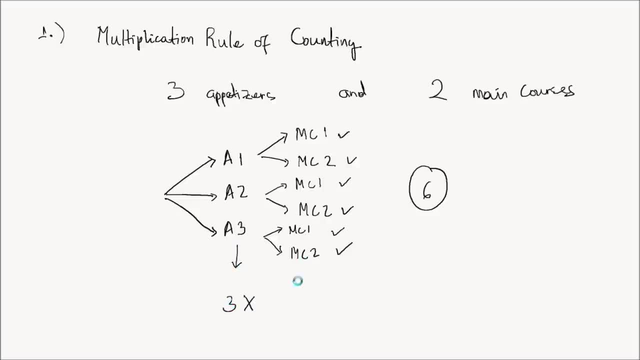 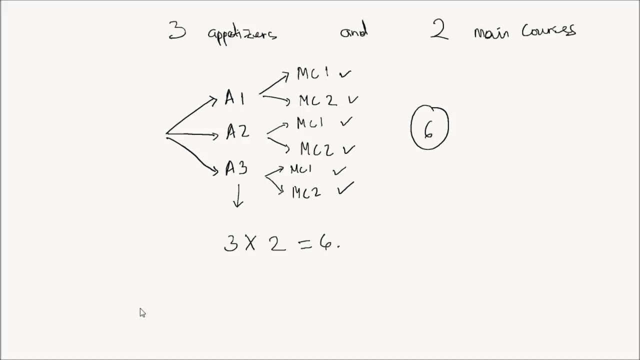 by the number of ways of choosing main courses, That is 2.. That gives you a 6.. That's a very simple example of multiplication rule of counting In general. if you have an experiment which has to be done in k different stages, that is stage 1, followed by stage 2, followed. 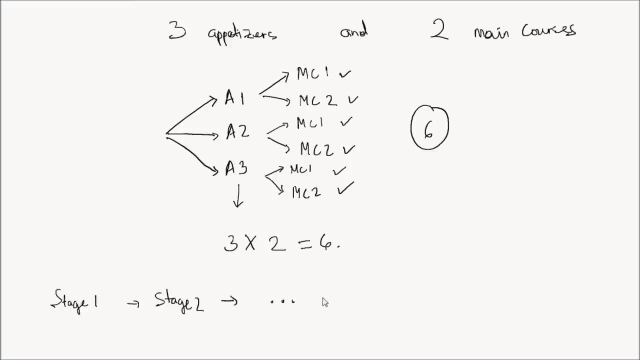 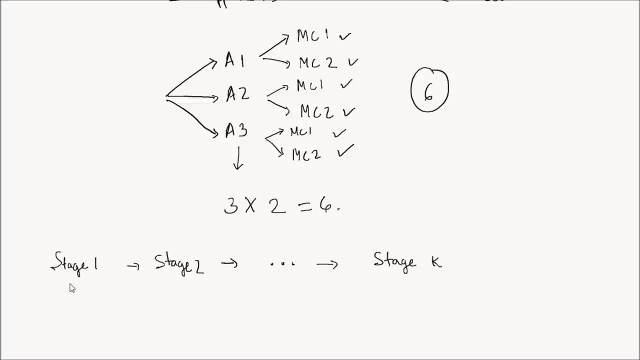 by stage 3,, followed by stage 4, and so on all the way up to stage k. And also, if you have n1 number of ways of doing stage 1, n2 number of ways of doing stage 2, n1 number. 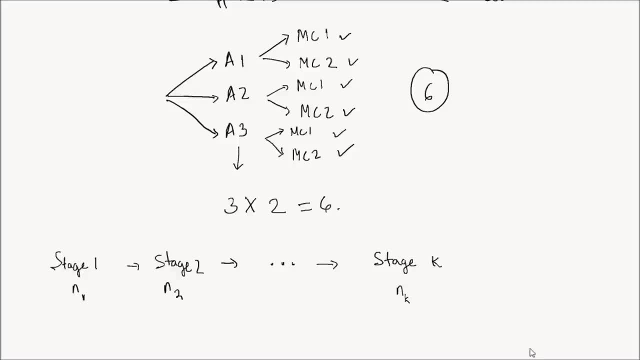 of ways of doing stage k, then the number of ways of doing the experiment or the number of all possible outcomes in the experiment is n1 times n2 times n3 times, all the way up to nk, And that is the multiplication rule of counting. Okay, Let's say we have an N. 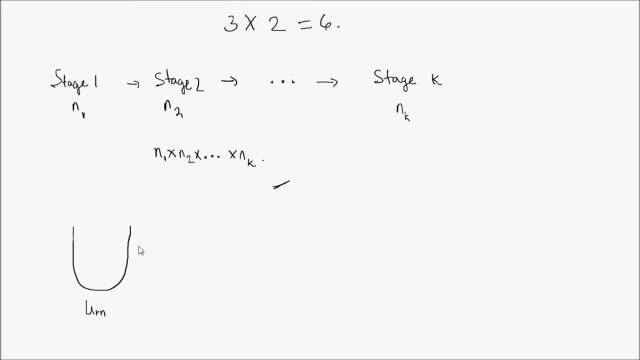 which contains 4 distinct marbles. To make them distinct, let's say we have one of them is red, one of them is blue, one of them is green and maybe one of them is black. Okay, Suppose you draw a marble from the urn. 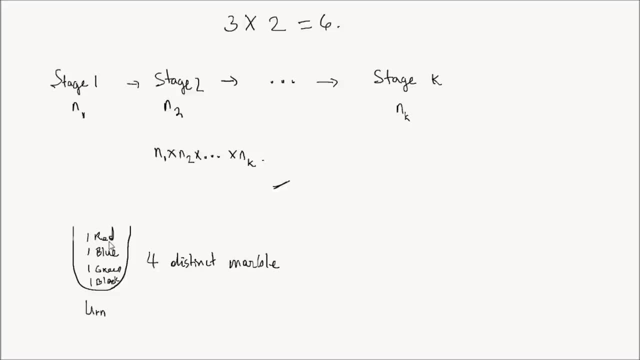 Replace it back into the marble after looking at what color it is, and then draw a second marble from the same urn. And how many ways can you do that? So we have two consecutive draws with replacement In your first draw. you have two consecutive draws. 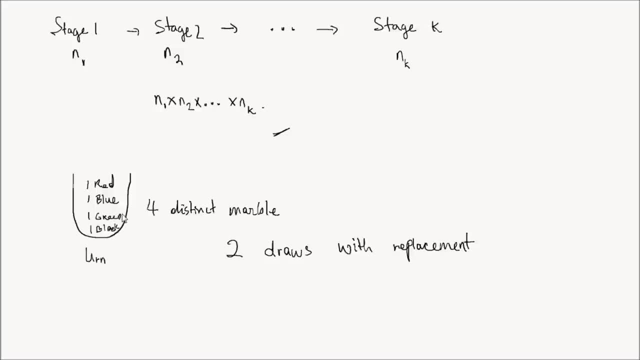 You have four different outcomes. You could have the red, the blue, the green or the black. The first draw has four different outcomes But since you replace back the marble, you again have four different possible outcomes in your second draw. By multiplication rule of counting the number of ways you can choose two marbles and the 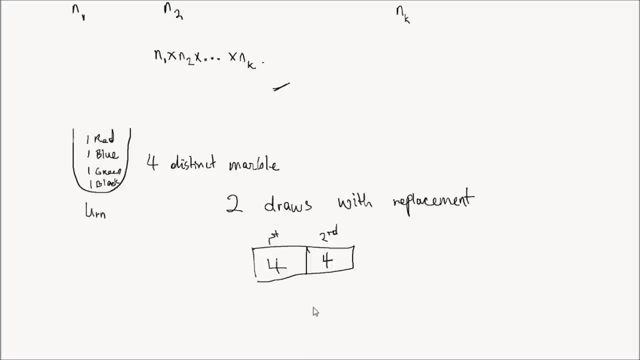 number of ways you can replace them one after the other with replacement is equal to 4 times 4, which is 4 squared. What if you change the sampling scheme somehow? Let's say, instead of replacing the marble back, you keep it aside, You don't put it back in, So you do two draws without replacement. 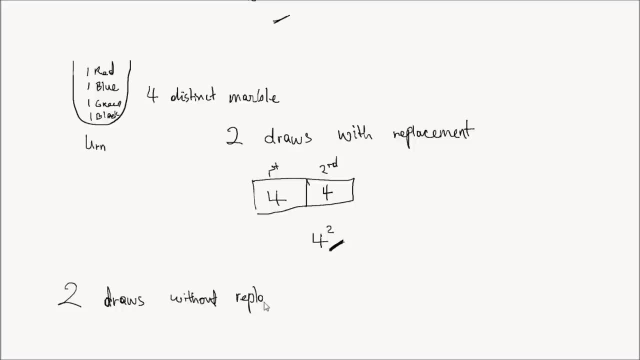 Okay, In this case you have, of course, for the first draw, you have four possibilities: red, blue, green or black. But for the second draw, since you don't put back the marble you had in the first draw, you only have three possible marbles to pick from. That is 4 times. 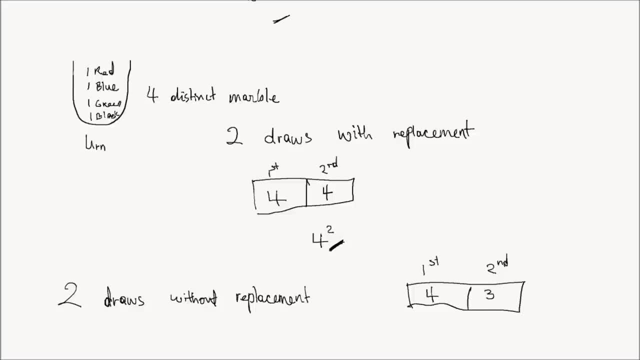 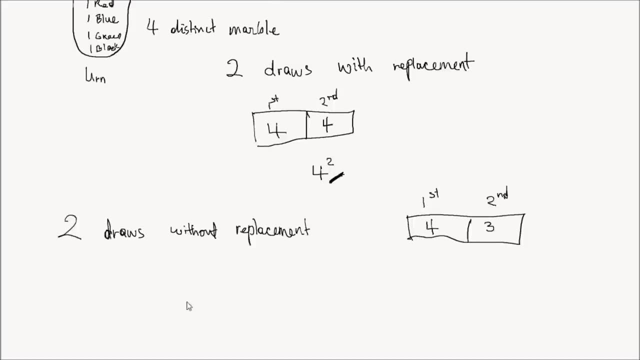 3,, which is 12.. Okay, Well, sometimes we ask the question: In how many ways can a series of k objects, Let's say, in how many ways can a series of k distinct objects? objects can be drawn from n distinct. 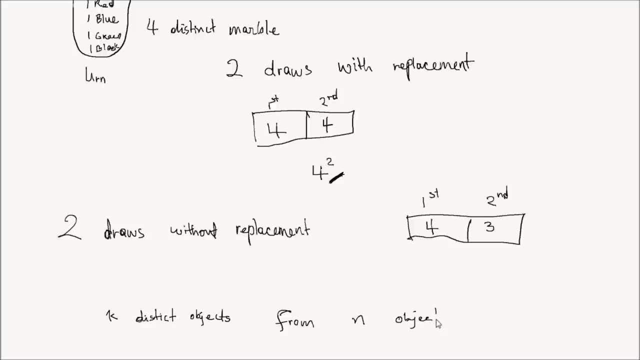 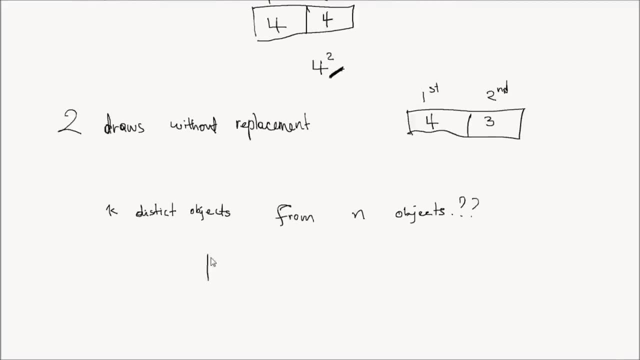 objects. Okay, Okay, In that case, the number of ways of doing that is equal to. for the first draw, you definitely have n possible distinct objects to pull from or to draw from. So there are n possible outcomes. But in the second draw, since you do not replace back the first draw, you're doing this without 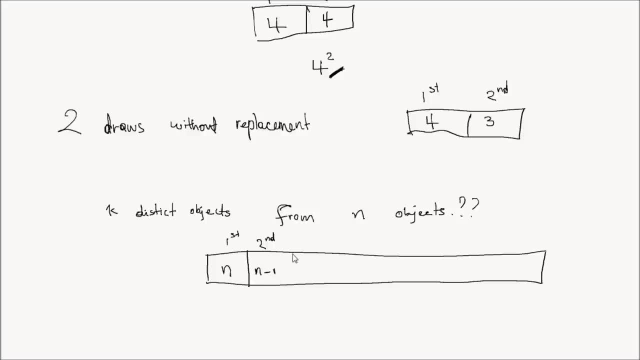 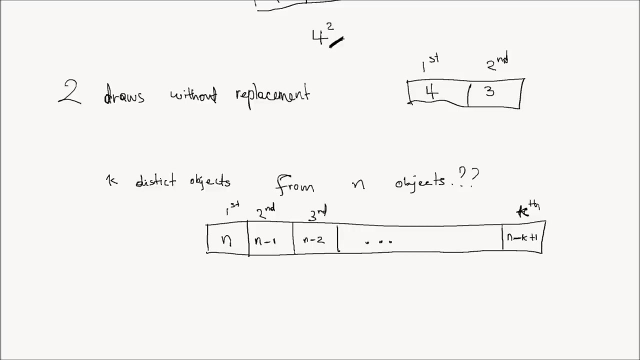 replacement. you have n-1 possibilities. The third one: you have n-2 possibilities And since we are drawing k draws in the kth draw, you have n-k-1 possibilities, The number of ways a series of k objects can be drawn. 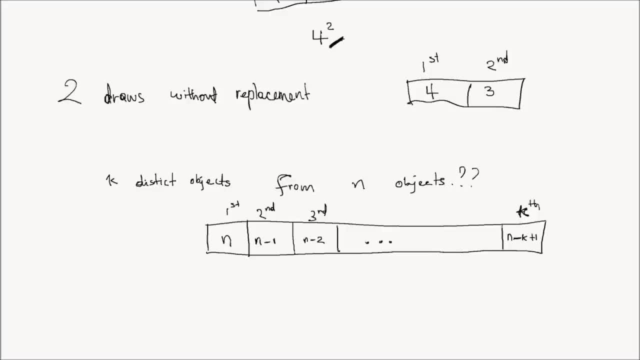 is equal to n-1 possibilities, Or it can be chosen from distinct n objects without replacement, as equal to n times n-1 times n-2 times, all the way up to n-k plus 1.. And when we do such kind of sampling we call this permutation. 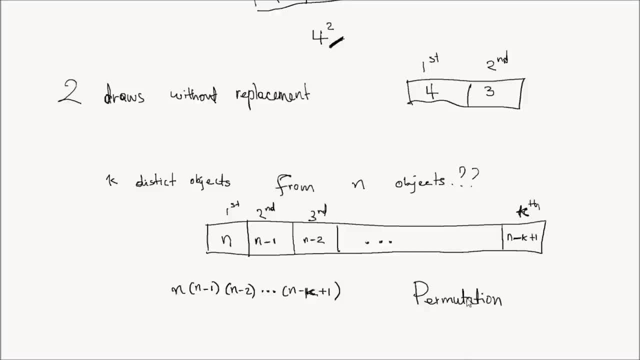 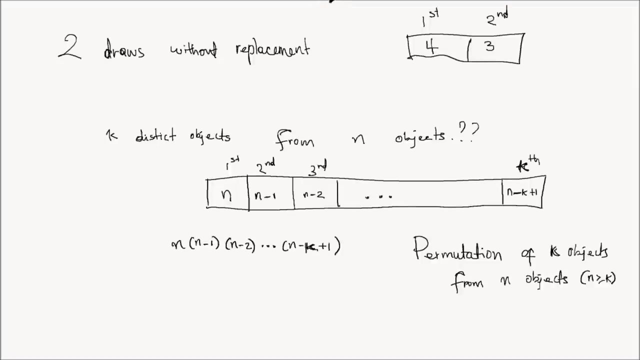 Or permutation of k objects from n objects. Permutation of k objects from n objects: Usually n is greater than or equal to k And it has to be greater than or equal to k And the notation we use for this permutation of k objects. 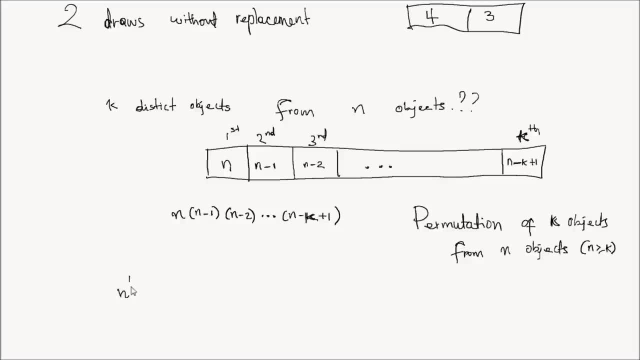 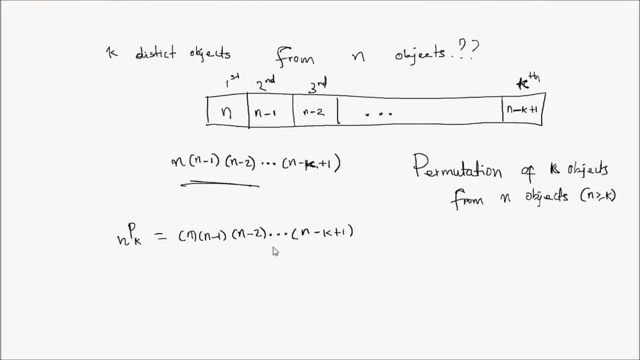 from n objects as n capital P k. And that is equal to, right here, n times n minus 1, times n minus 2, times n minus 3, all the way up to n minus k plus 1.. And this product can be written as n factorial divided by n minus k factorial, n P k, where I assume you know. 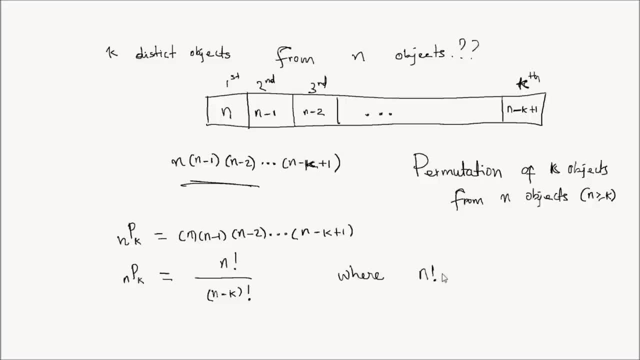 this, but I am going to write it anyway: n factorial is equal to n times n minus 1, times n minus 2, times n minus 3, all the way up to 2.. Okay, times 1.. By notation, 0 factorial is equal to 1.. Of course, 1 factorial is 1, 2 factorial. 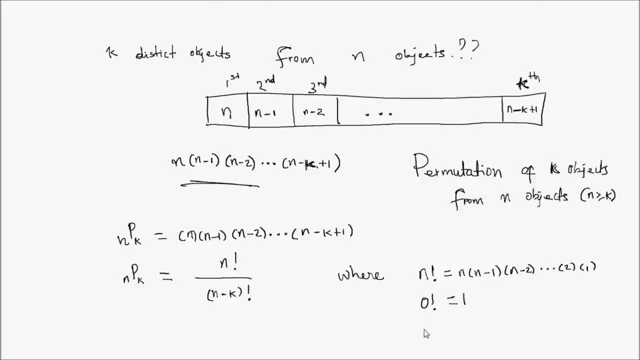 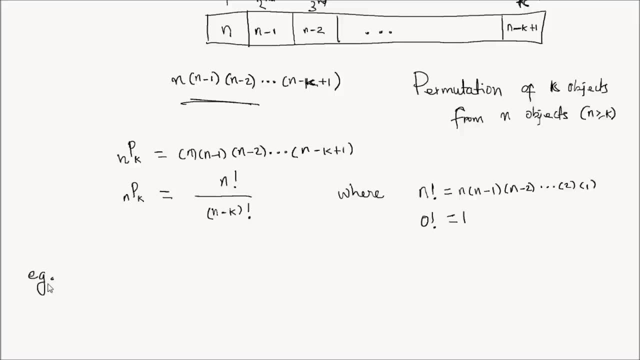 is 2,, 3, factorial is 6, and so on. Example: suppose there are 10 athletes competing in 100 meters run. So I have 10 athletes competing in 100 meters, And in how many ways can the rankings be assigned to the top 3 competitors? I would like to assign rankings to the top. 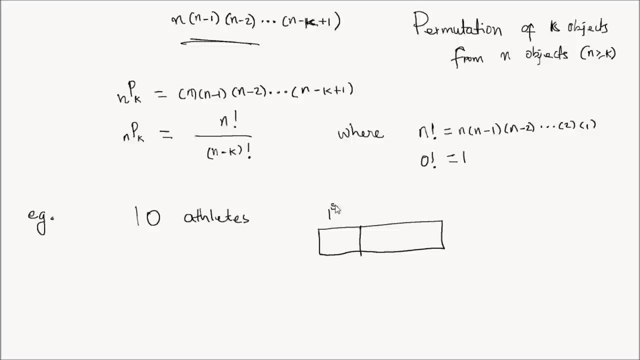 3 competitors: First position, second place and third place. I have 10 athletes competing in 100 meters run. So I have 10 athletes competing in 100 meters run, So one of the 10 would cross the line first, Right after he crosses there. 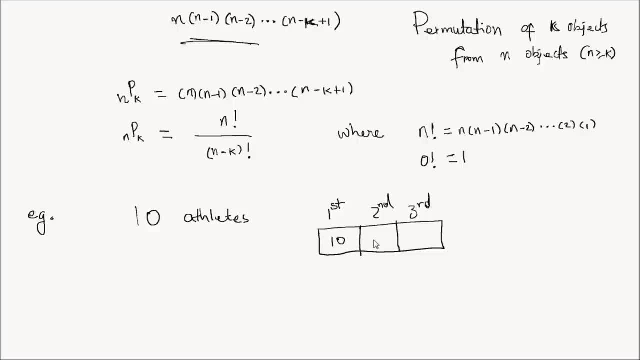 are 9 left to cross the line. So I have 9 possible competitors to be number 2.. And then I have 8 possible competitors to be number 3, because the first 2 have crossed the line already. So the number of ways of assigning rankings. 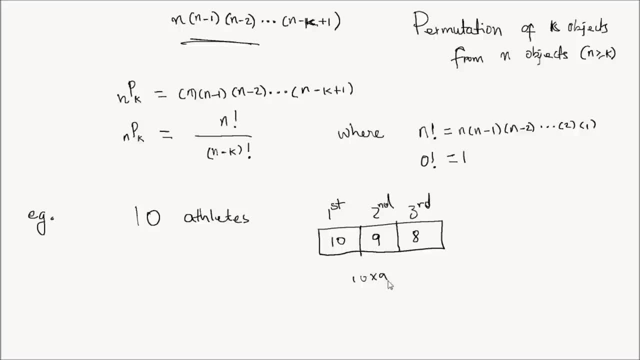 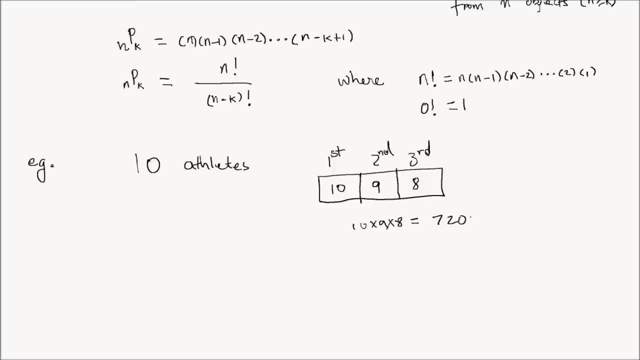 to the top 3 is 10 times 9 times 8. And that is, I think, 720.. But one thing I want you to note here is that the ordering of the rankings matters And permutation order matters. By the way, the 720 is permutation of 3 objects. 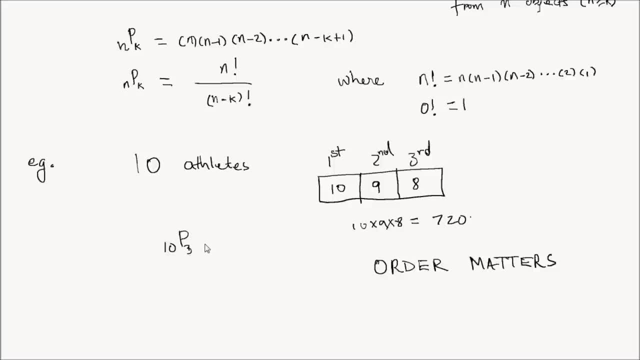 So I have 10 objects from 10, which is 10 factorial divided by 10 minus 3,, which is 7 factorial, Which is 10 times 9 times 8 times 7 factorial divided by 7 factorial, So that 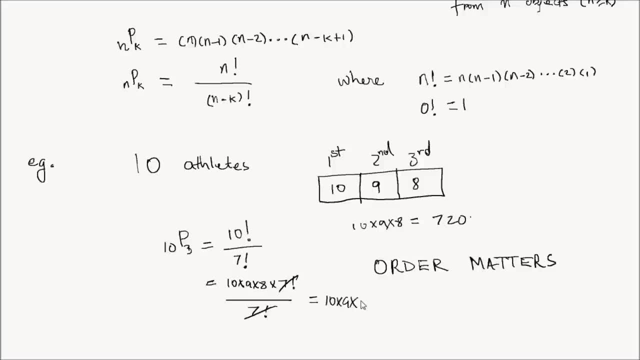 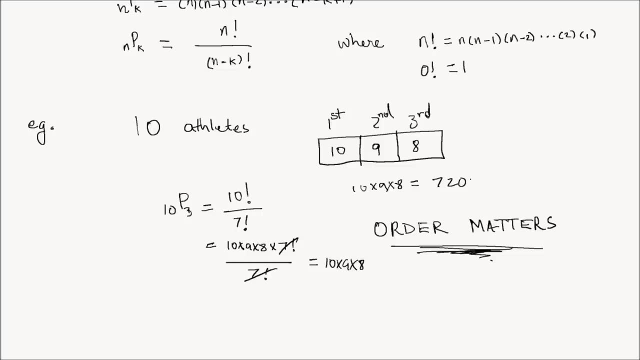 cancels out, And I have 10 times 9 times 8, which is 720.. Why do I say the order matters here? Well, the reason is remember that in 2012 Olympics in London, I think Usain Bolt came. 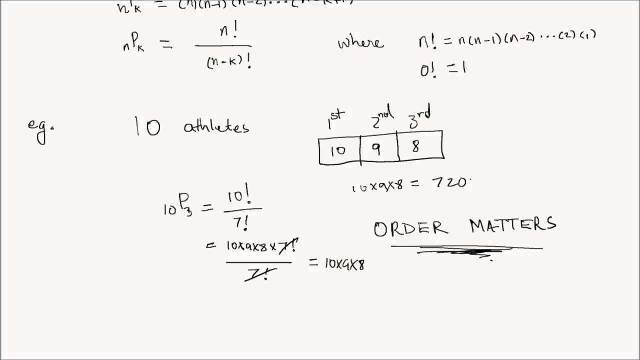 first and Johan Blake came next. The third one is the American Justin Gatelin. So Usain Bolt first and Johan Blake next is a completely different ordering from Johan Blake first and Usain Bolt second, And the reasons for that are basically these. So let's move on to the second order. So here's. 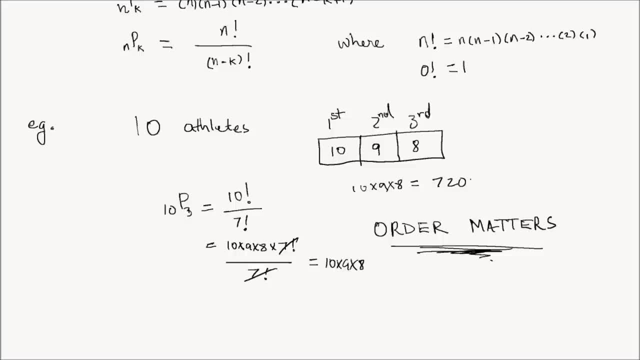 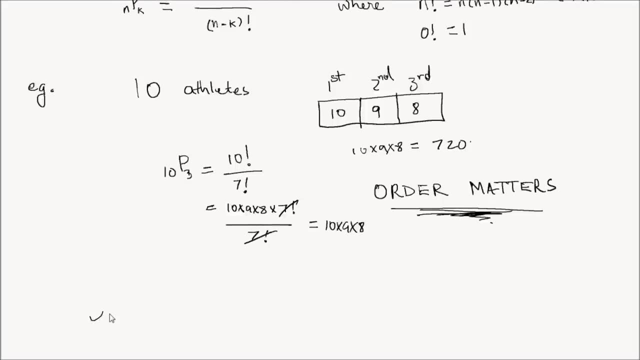 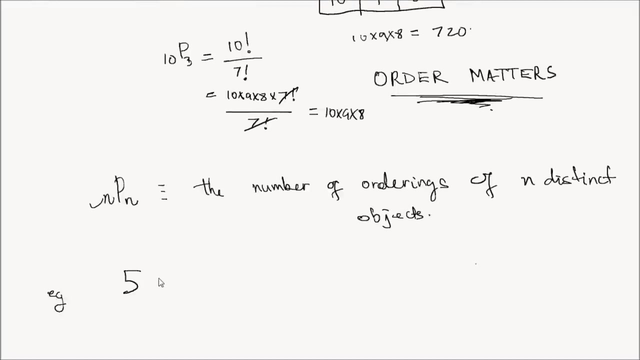 So the ordering matters here and permutation, And also if I do the permutation of n objects from n possible objects, I am finding the number of orderings of the objects Of n objects. Let me give an example here. Suppose we have five books which are distinct. You can tell. 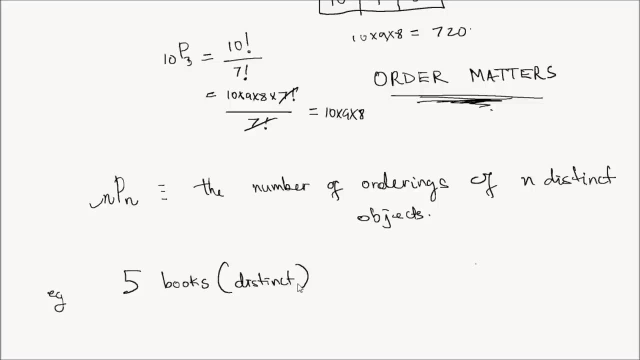 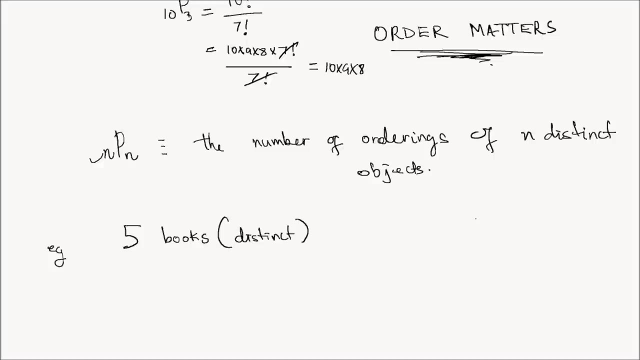 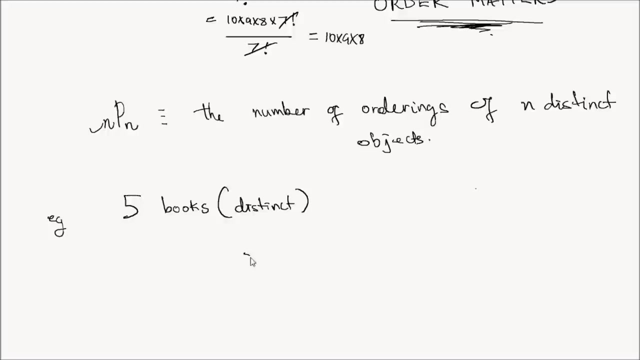 one from the other. maybe the first one is chemistry book and the next one is math book and the third one is… biology book and so on. Five different, completely distinguishable books, And how many ways can I arrange them on a bookshelf? The number of ways of arranging this on a bookshelf is five. 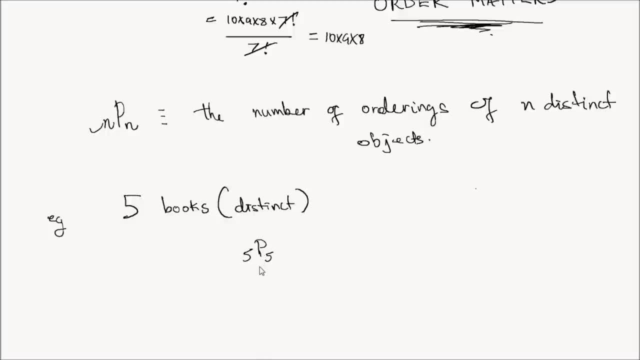 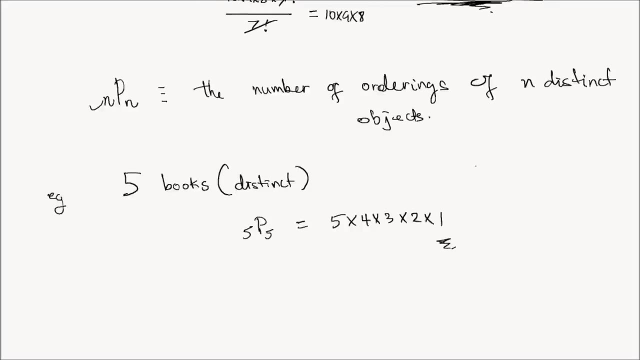 permutation five: Permutation of five books from five. That is equal to five times four times three times two times one. Let me give it a twist here. What if, let's say, two of the five books are completely identical, That is, you cannot tell one from the other? Again, I have five books. 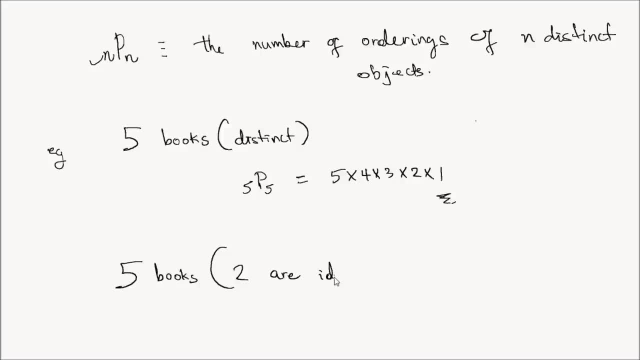 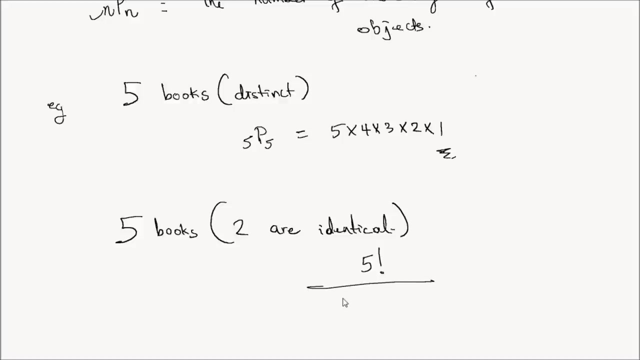 Two are identical. How many orderings of the five books do I have on a bookshelf? And the answer to that is five factorial divided by two factorial, which is five times four times three. Okay, In general, in general, if I have n objects. 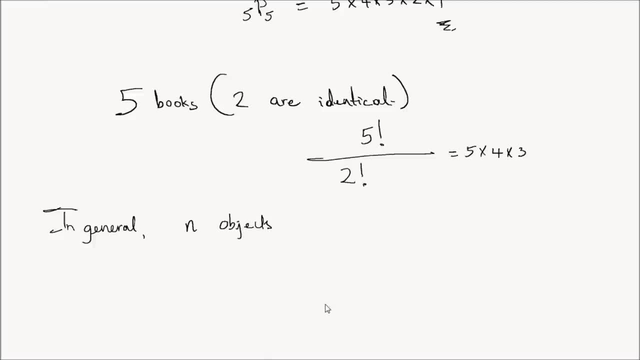 let's say I have n objects, or I can think of them as n marbles or n books, and let's say n1 of them belong to one group, Let's say they are red marbles And maybe n2 of them are blue marbles, And you cannot tell one from the other. 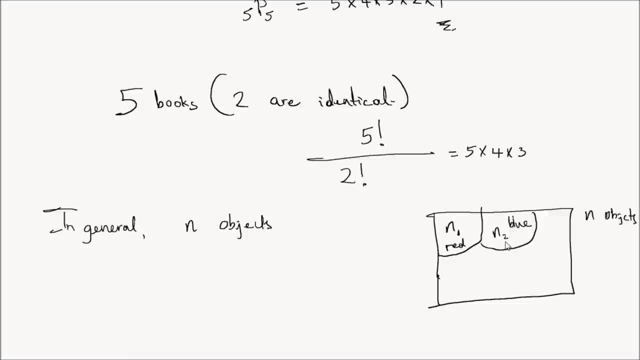 If you're looking at those n2s- Okay And maybe n3 of them are again green, They cannot be told apart. So let's say we have k different partitions, So nk of them belong to a partition or a group that are completely identical. 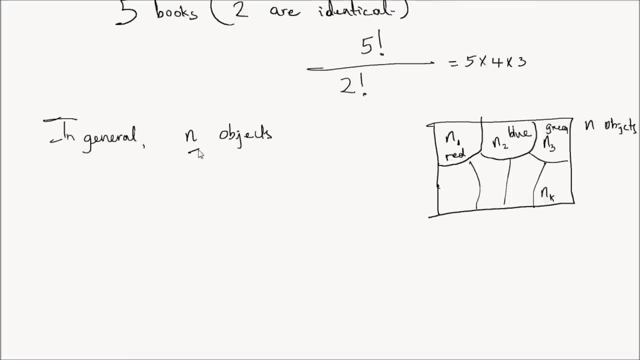 Then the number of ways of arranging those n objects with such property is the following: Note that n is equal to n1 plus n2 plus n3, all the way up to nk. Okay, The number of ways of arranging those n objects is n factorial, divided by n1 factorial times n2 factorial times n3 factorial. 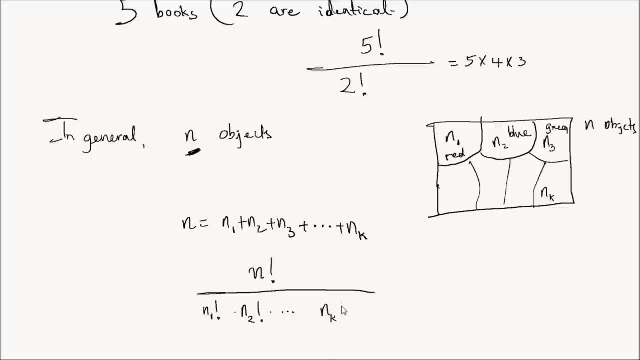 And the denominator is: n1- factorial times, n2- factorial times, n3- factorial. And the denominator is: n1- factorial times- n2- factorial times, n3- factorial. And the denominator is: n1- factorial times, n2- factorial times, n3- factorial. all the way up to nk- factorials. 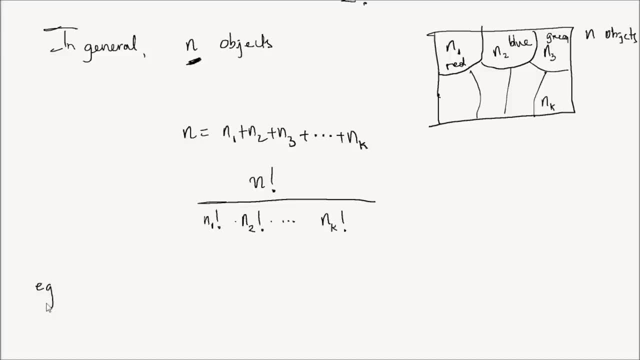 Okay, A very good example, which is typically used, is the number of ways of arranging the letters in the word Mississippi. Let me write it down: M-I-S-S-I-S-S-I-P-P-I, Mississippi, And how many ways can you arrange the letters in the word Mississippi? 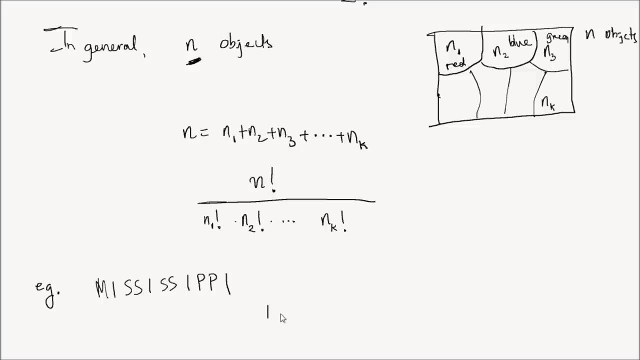 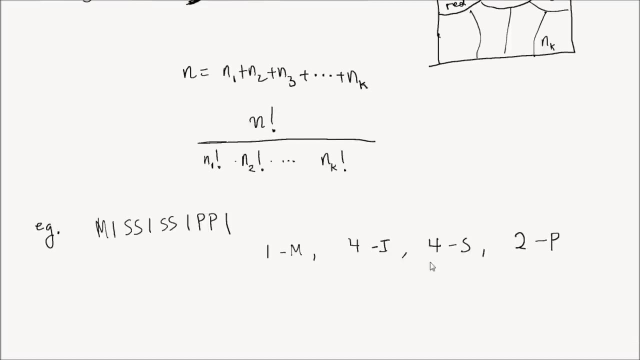 So in this word I have one M, four I's again, four S's and two P's. One plus four plus four plus two, that's eleven. So I have eleven letters to arrange, Of which one is an M and four are completely identical.